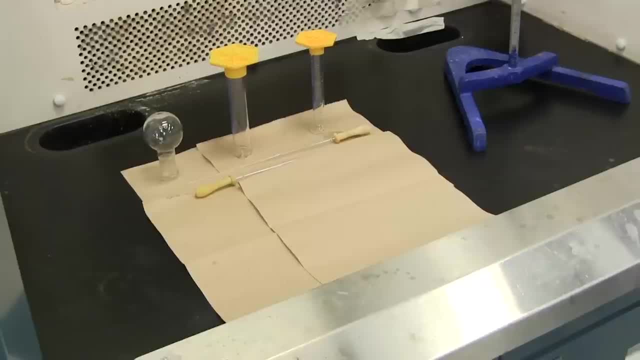 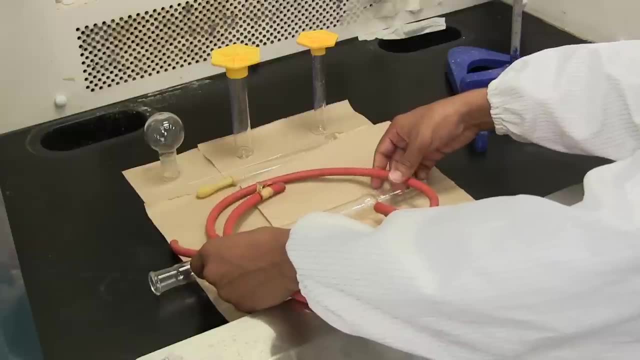 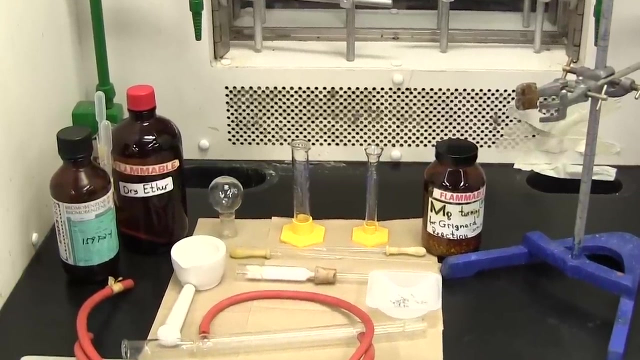 Once you have rinsed the glassware with acetone, invert them onto paper towels and set them aside to dry for roughly 10 minutes to remove any residual acetone which can cause unfavorable side reactions. Refer to your lab manual for a description of the side reactions that can occur if the preparation of the Grignard reaction is contaminated with water. 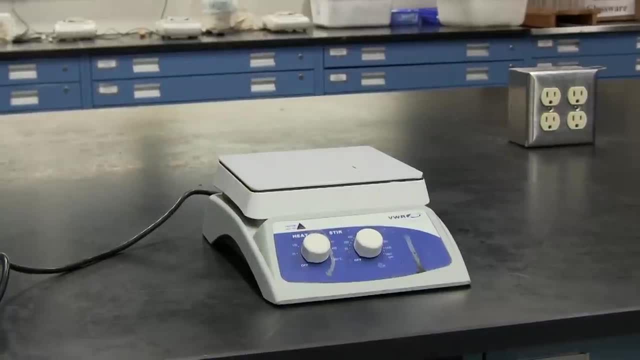 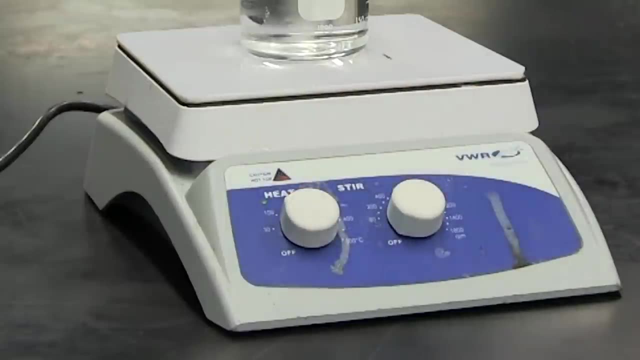 While the glassware is drying, set up a hot plate on the bench outside the fume hood, since the ether must be kept away from the glassware. Heat a 200 ml beaker of water on the hot plate until it is warm. Do not heat until boiling. 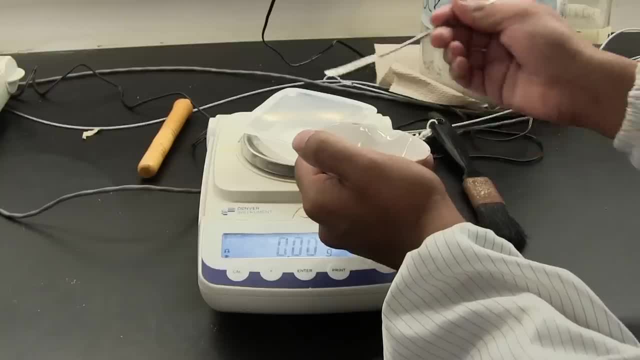 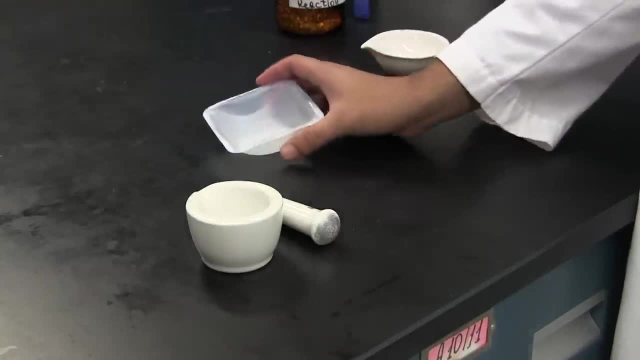 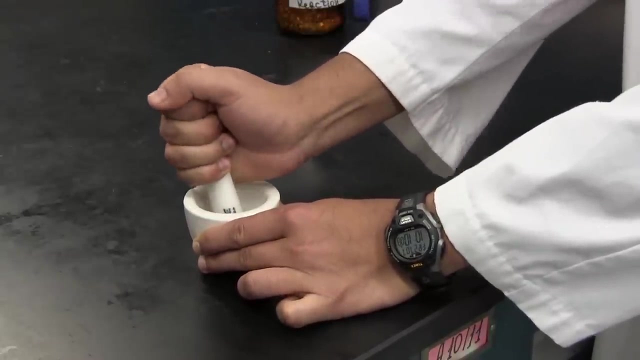 Use a weighing boat to obtain the required mass of magnesium turnings. Transfer the weighed out magnesium shavings into the mortar for grinding Thoroughly. grind the magnesium turnings with the mortar and pestle. This is an important step as it exposes more surface area of the magnesium for the reaction to take place. 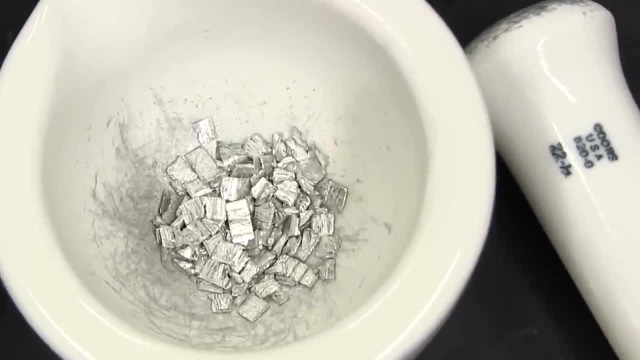 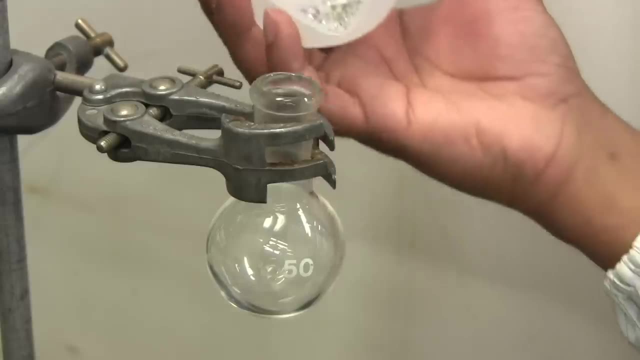 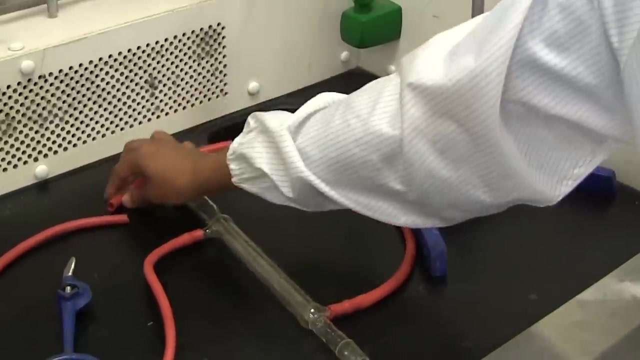 This is what your ground up magnesium turnings should resemble. Attach the 50 ml round bottom flask to the retard stand and place the magnesium turnings inside. Here is a condenser. The bottom pipe is connected to the tap and the upper pipe is connected to a ring clamp which is placed on the sink. 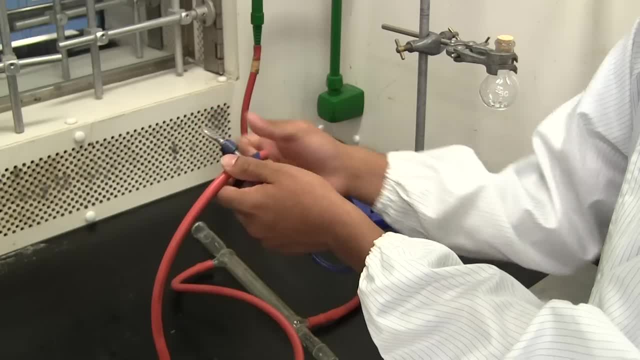 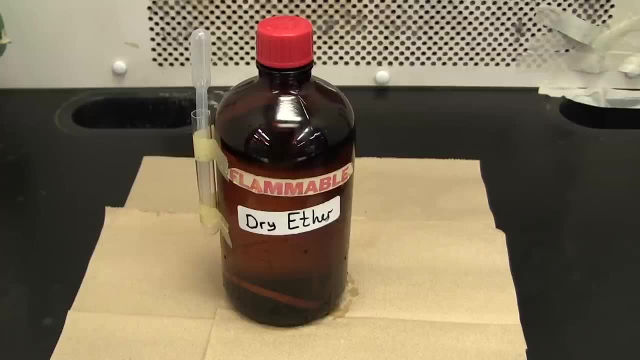 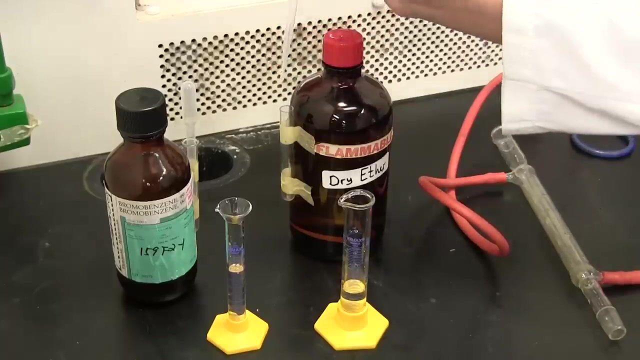 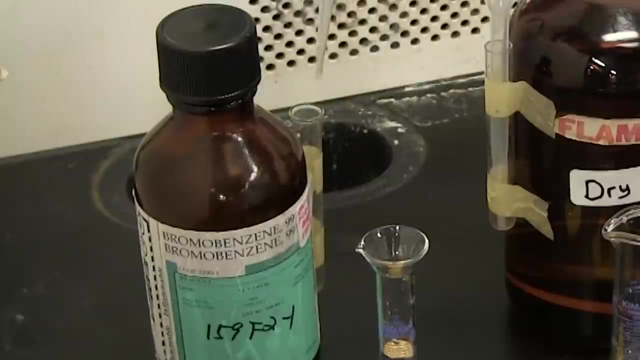 Ensure that there is a steady flow of water. Here is a bottle of dry ether. This will be utilized as our solvent To ensure that the ether is dry. look at the sodium ribbon and ensure that it shines. To prepare a feeding solution, add the required amount of dry ether and halogen compound separately, using different pipettes within a graduated cylinder. 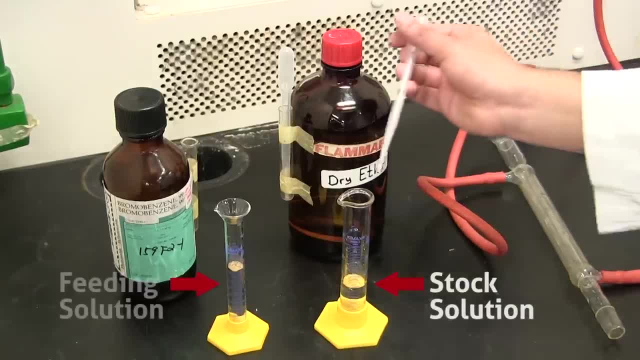 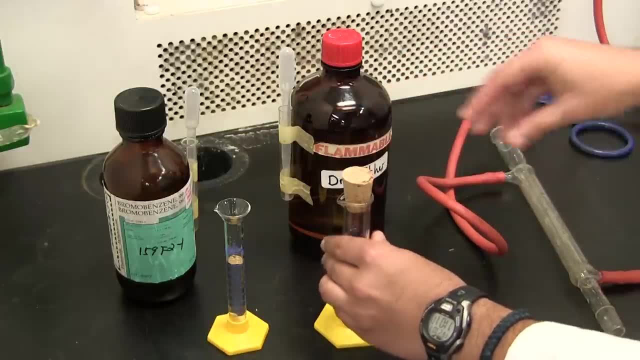 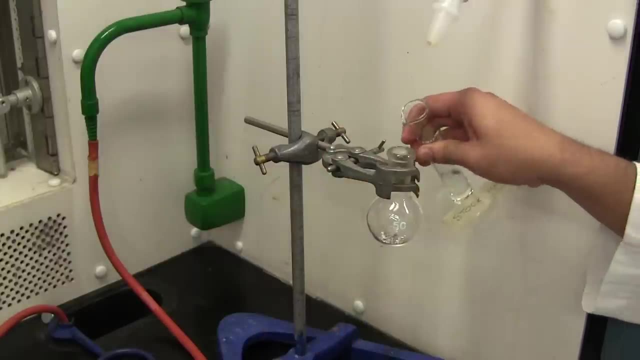 Here is a stock solution along with the feeding solution. Prepare the stock solution using the required amount of dry ether and halogen compound solutions. Ensure that you cork the graduated cylinder so that the solution does not evaporate. Once you have both solutions prepared, transfer the stock solution into the round bottom flask and quickly attach the condenser to it. 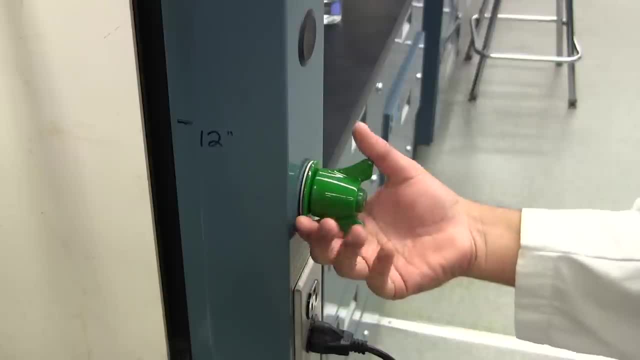 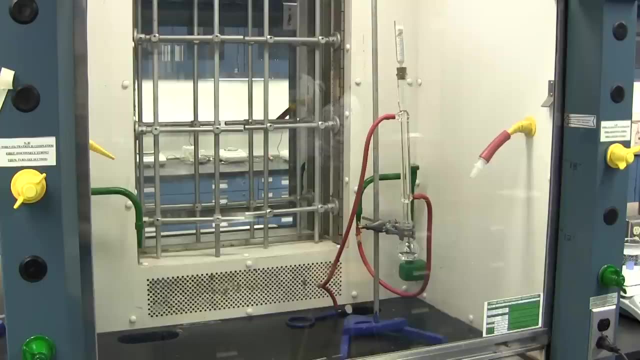 At this point you should start the water flow. Here is the experimental setup that will be used for the preparation of the Greenyard reaction. The round bottom flask will be the site of reaction. The condenser will ensure that all the volatiles can flow. 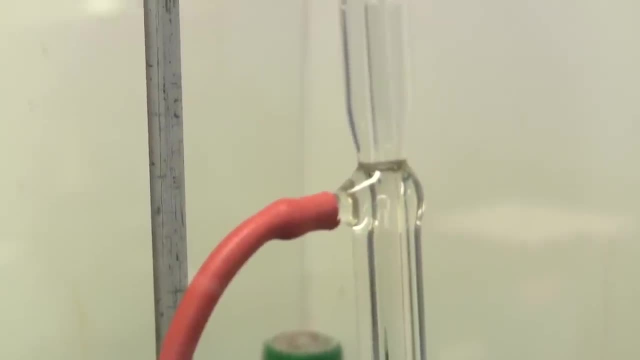 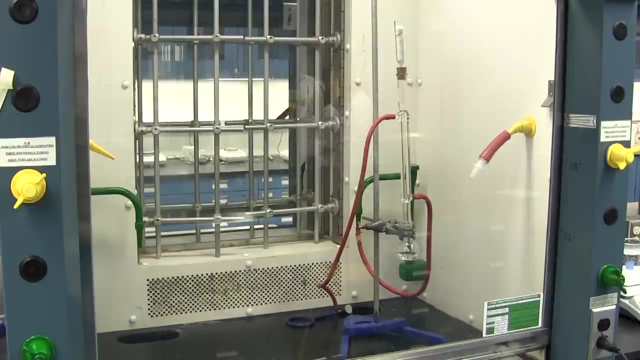 All the volatiles can be reused in the mixture, and the drying tube has been employed such that no moisture is incorporated in the reaction. While working on any experiment, please ensure that the fume hood is placed at the maximum height of 18 inches. 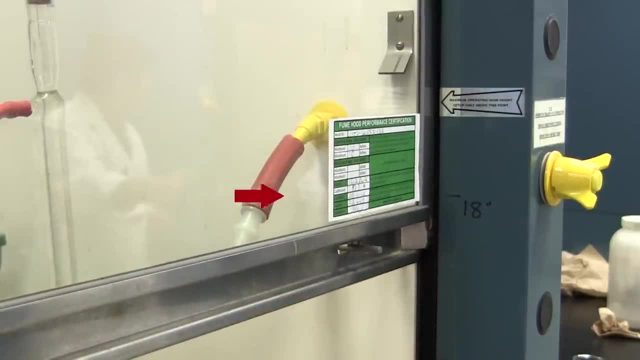 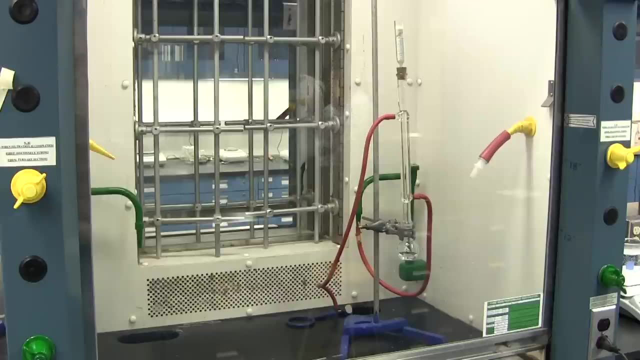 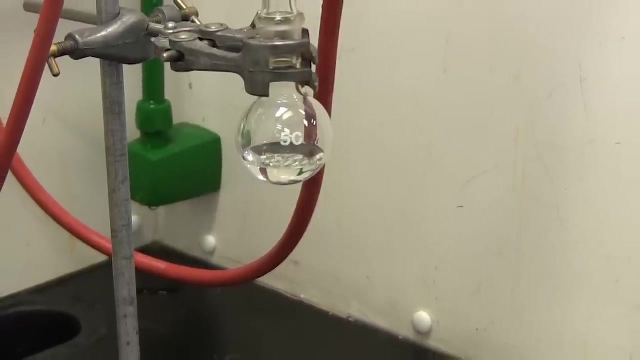 As per lab safety requirements, a height over 18 inches is restricted and is not considered a safe practice. The Greenyard reaction is a self-sustaining reaction Once it is initiated by a source of heat. Bear in mind that the heat source must be subtle. 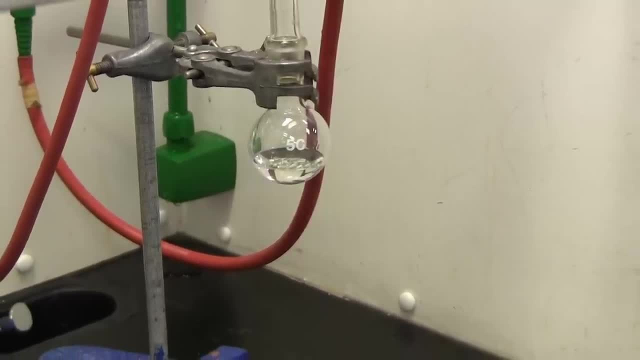 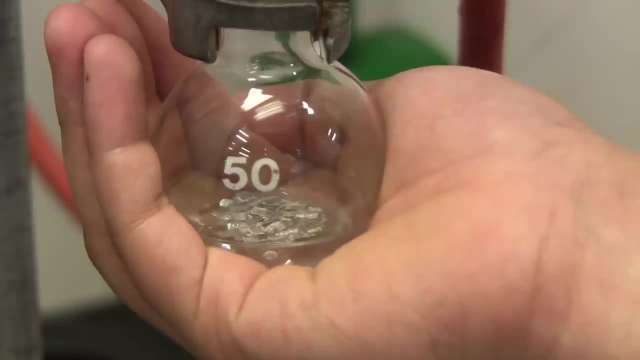 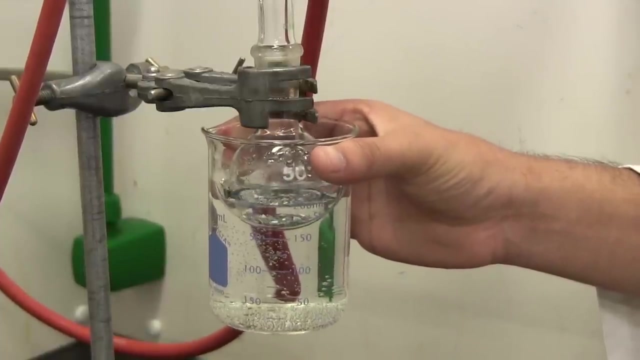 The source should be warm enough to initiate the reaction, but also ensure that it does not produce any side reactions. Initiate the reaction by using the heat of your palm. If you cannot start the reaction using your palm, you can employ a warm water bath to initiate the reaction. 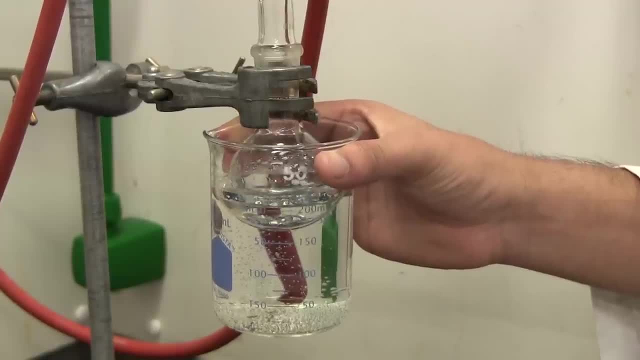 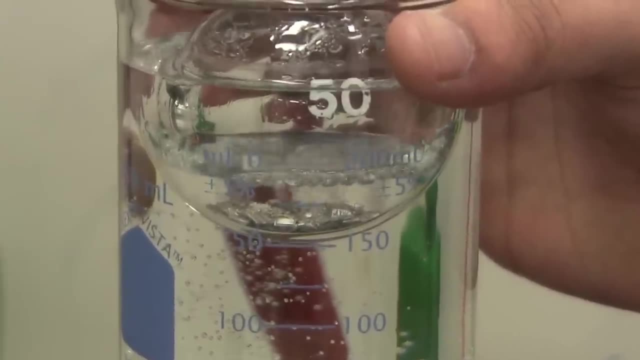 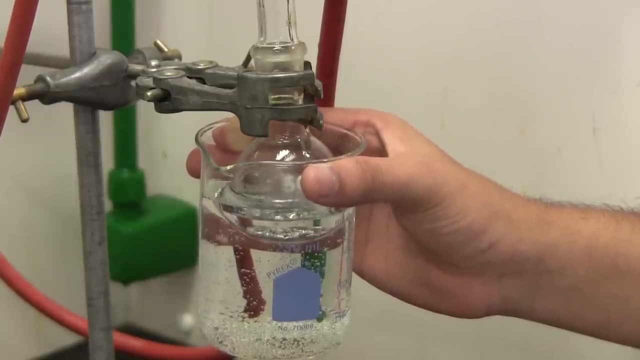 This is a warmer source of heat and provides a uniform distribution as well. The reaction mixture now appears to bubble, indicating the transfer of heat. The beaker is removed when the reaction is proceeding vigorously. See whether the reaction is self-sustaining or whether the solution turns from colorless to gray. 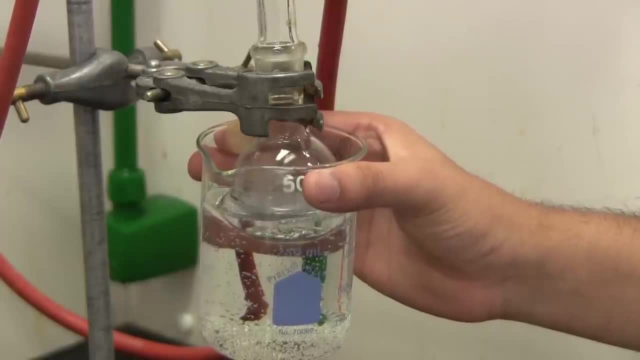 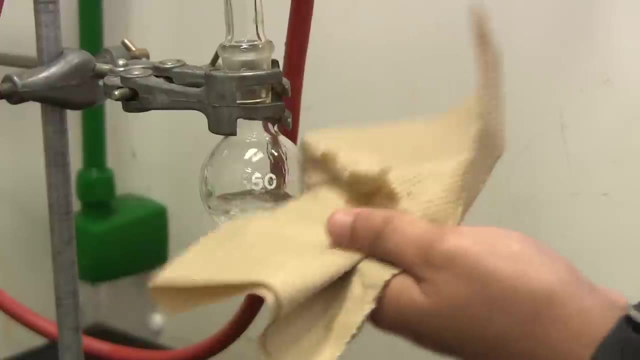 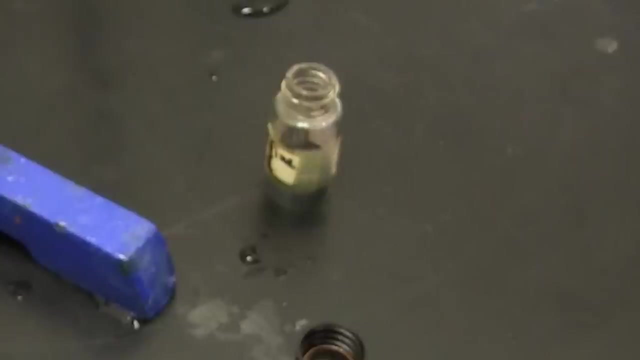 Once you remove the warm water bath and observe that the reaction is self-sustaining, dry the bottom of the flask using a paper napkin. The solution should appear colorless at this point. Here is a bottle of iodine crystals. If you are unable to initiate the reaction using the previous techniques mentioned, these crystals can be used to initiate the reaction. 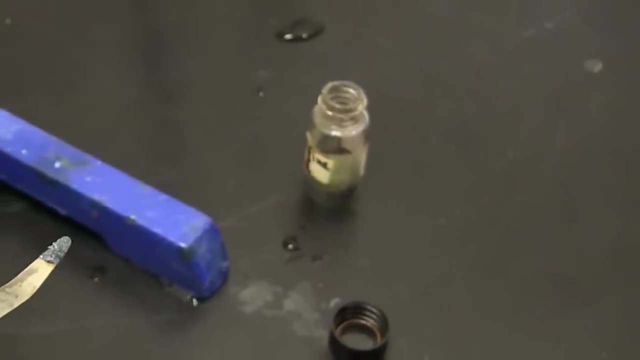 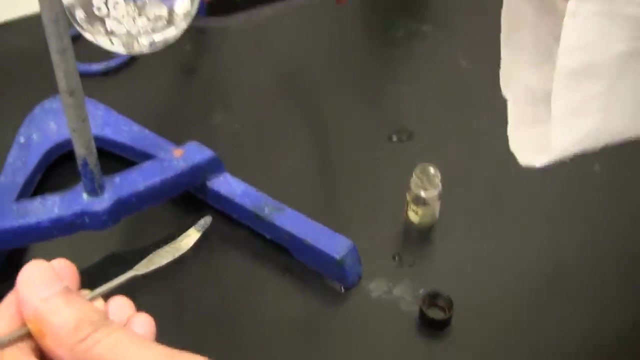 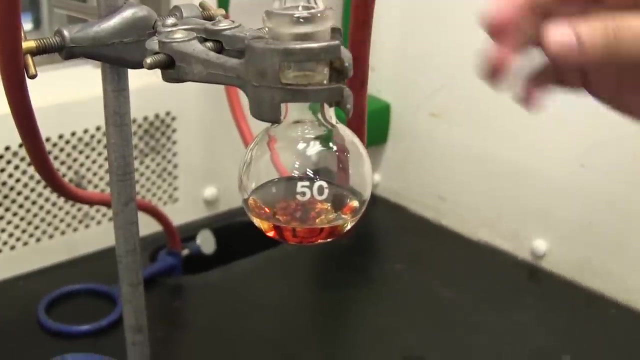 The iodine replaces the halide from our halide compound and this facilitates the reaction. to initiate: Obtain the crystals using a scupula so that the tip of the scupula is covered. Transfer the iodine crystals to the reaction mixture. Immediately add the crystalline.